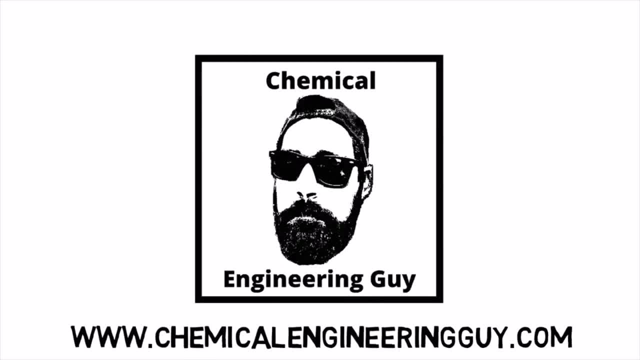 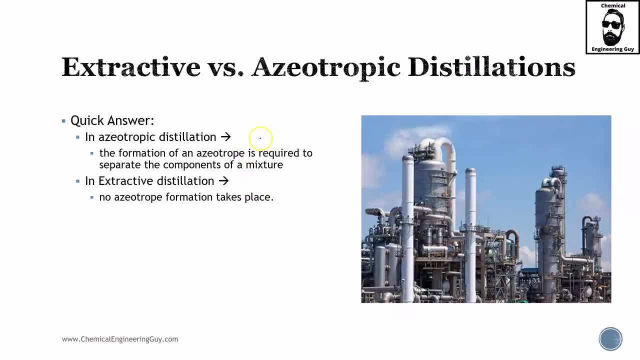 So, now that we know about the extractive and azeotropic distillations, let us make a clear difference between both of them. Now, of course, both are distillations, meaning that the main idea is that they exploit the difference in volatility between the components that we 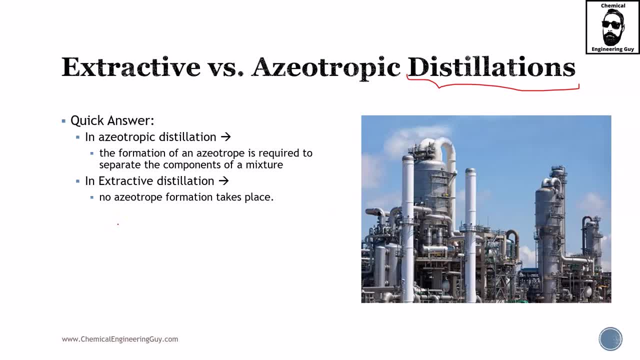 want to separate. Now, the quick answer of the difference is that in azeotropic distillation we most form, or the formation of an azeotrop is required to separate the components of the mixture. Now, as you can see, azeotropic formation here, as the name implies, is the main issue. 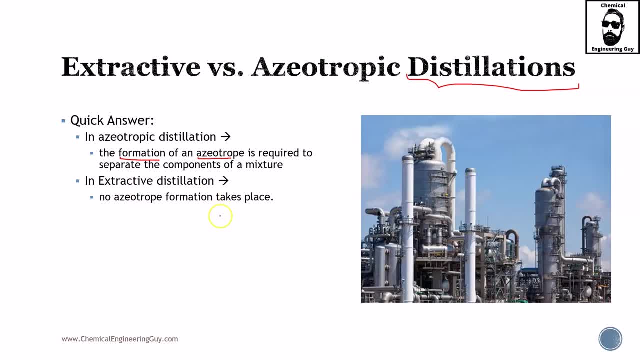 Now, in extractive distillation, we don't need to form an azeotrop. Actually, what we're going to do is just to add a material and this is going to be azeotropic distillation. Now, in extractive distillation, we don't need to form an azeotrop. 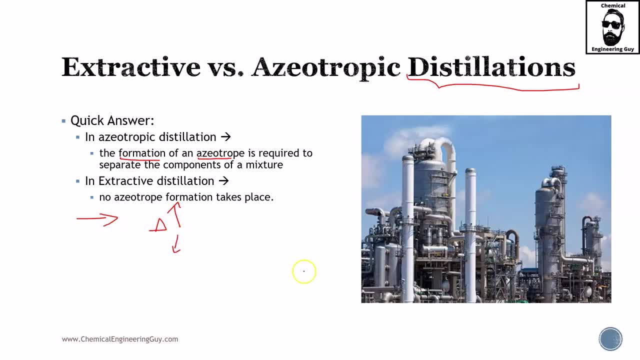 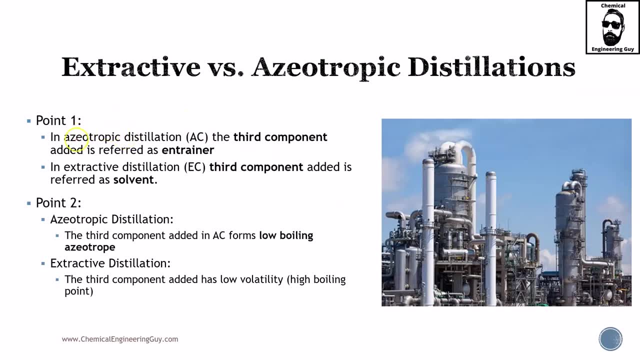 Theoretically improving the separation coefficient due to the volatility differences. Now let us make it even clearer. Point one: in azeotropic distillation the third component added. the MSA that we're adding is referred as the entrainer In extractive distillation. the third: 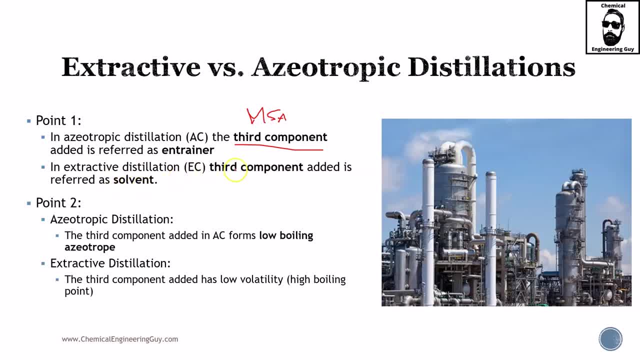 component added is referred as the solvent. Now, both of them are external materials which in theory will be recovered and is not part of our final product. Point number two: azeotropic distillation. the third component added by the azeotropic distillation procedure will have or yield: 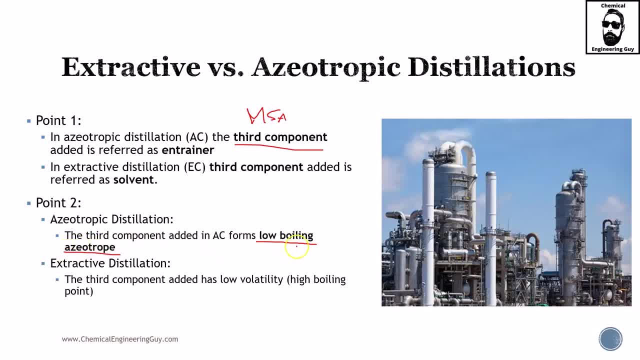 a low-bowling azeotrop or low-bowling point. azeotrop Extractive distillation, on the other hand, will not have a bowling point. Actually, the reverse is true: It's going to have a very high. 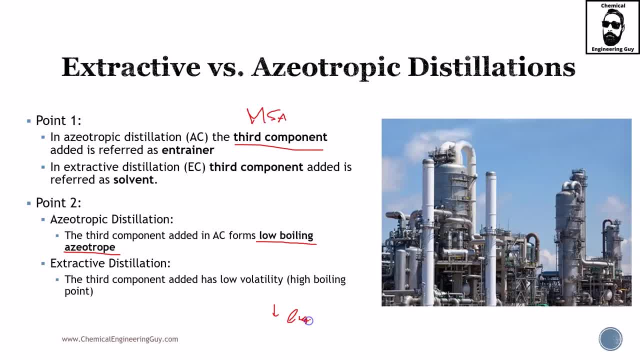 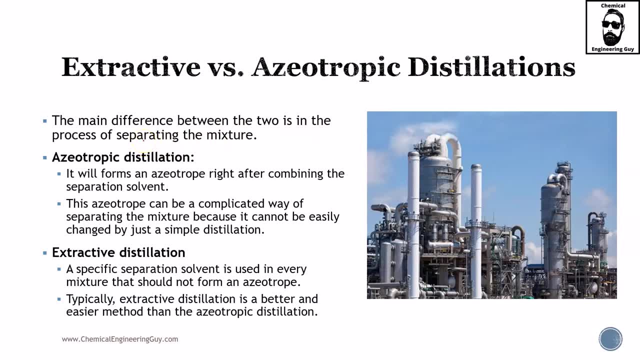 bowling point, Because we want this to remain as a liquid. The main difference between the two is in the process of separating the mixture as well. Azeotropic distillation will form an azeotrop right after combining the separation solvent. This was already addressed. The azeotrop can be a complicated way. 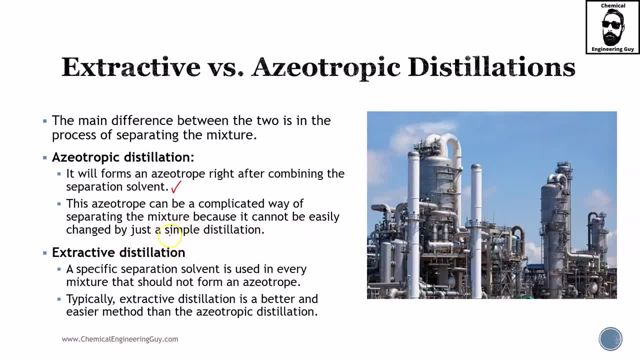 of separating the mixture, because it cannot be easily changed by just a simple distillation. Now, as you can imagine, azeotropic distillations can get a little bit more complicated. So we're going to have a very high bowling point. So we're going to have a very